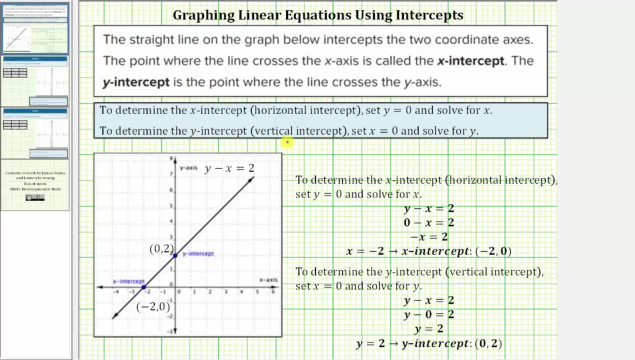 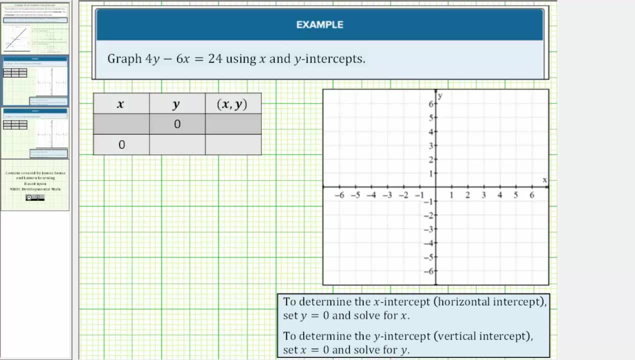 In general, to determine the y-intercept or vertical intercept, we set x equal to 0 and solve for y Again. this should make sense because any point on the y-axis or vertical axis has an x-coordinate of 0.. Going back to our example, another way to find the intercepts would be to complete this special table of values where, for one row, y is equal to 0.. For the second row, x is equal to 0.. 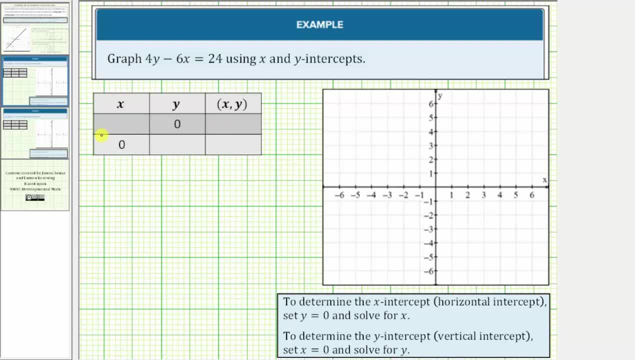 So let's begin by completing this first row, Which will give us the x-intercept. Remember, in general to determine the x-intercept, we set y equal to 0. So if we set y equal to 0 in our equation we would have 4 times 0, minus 6x equals 24.. Simplifying this would be 0. So we have negative 6x equals 24.. Divide both sides by negative 6.. 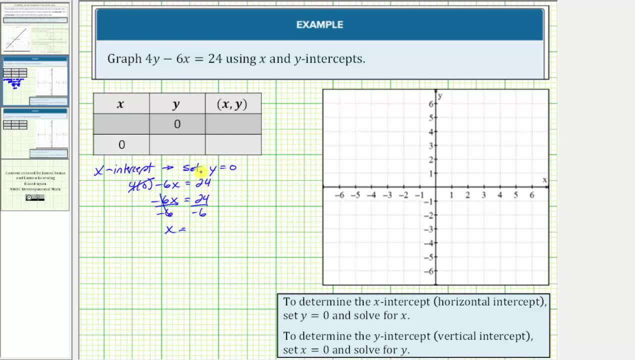 Simplifying, we have x equals 24, divided by negative 6 equals negative 6.. Simplifying, we have x equals 24, divided by negative 6 equals negative 6.. So we have negative 4, which gives us the x-intercept or horizontal intercept, negative 4 comma 0.. 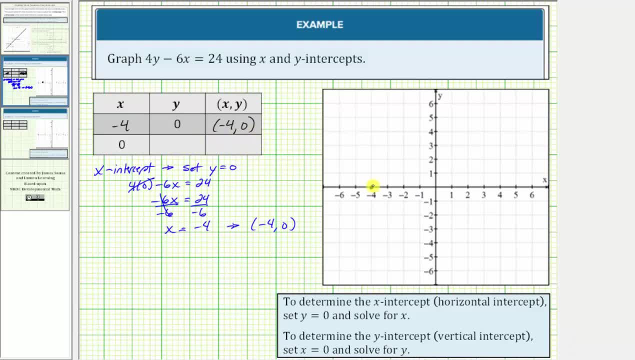 Let's go ahead and plot this point on the x-axis, which would be this point here And now. let's find the y-intercept by completing the second row of the table. So to find the y-intercept, we set x equal to 0 and solve for y. 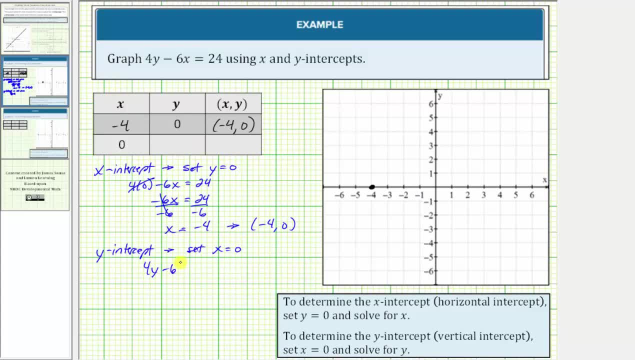 If we set x equal to 0, we have 4y minus 6 times 0 equals. 4y Minus 6 times 0 equals 24.. Simplifying, we have 4y equals 24.. Divide both sides by 4. We have y equals 6, which means the vertical intercept or y-intercept is 0 comma 6.. 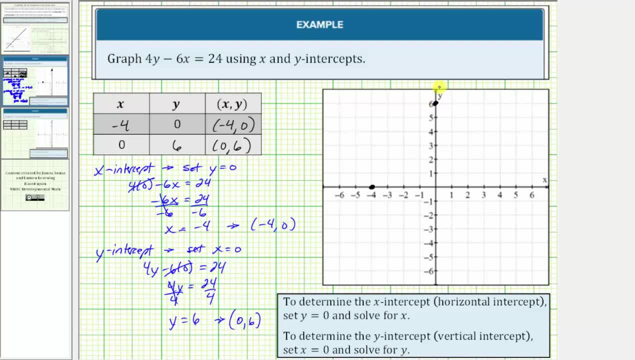 Let's go ahead and plot the point 0, comma 6, which would be here. Now that we have the intercepts, we can graph the line. This is the line. 4y minus 6x equals 24.. Let's look at a second example.